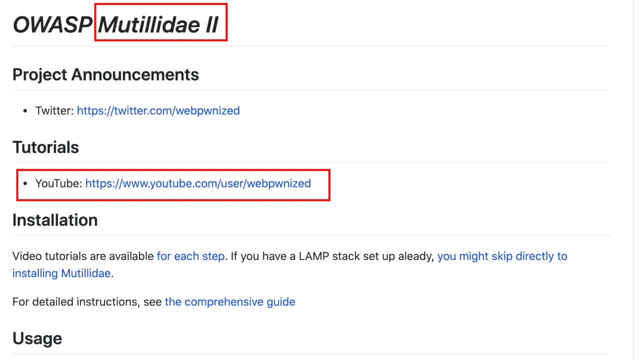 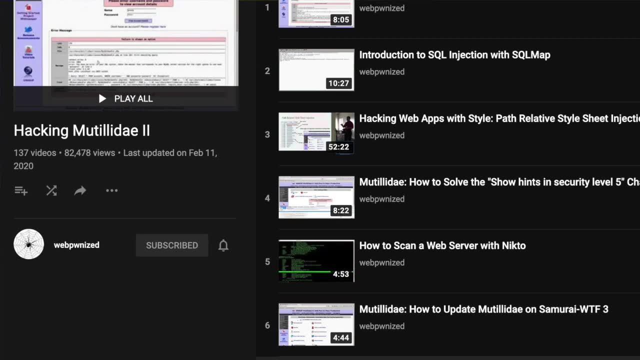 incorrectly. I found that the group that actually developed this platform has their own YouTube channel with tons of videos on how to install it, had used it, how to learn from it, And I really thought that that would just be kind of redundant and duplicative for me to do it. 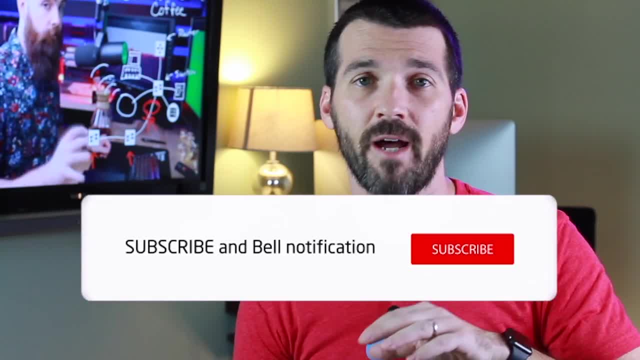 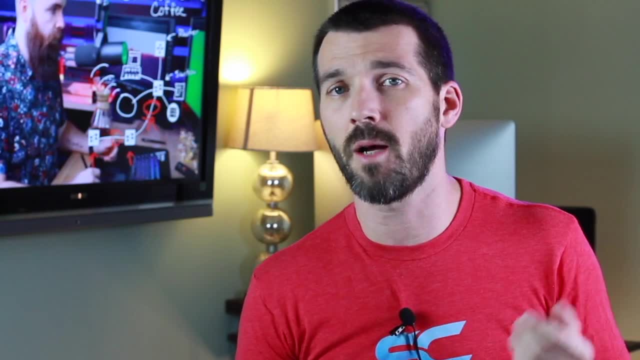 So I'll link in the show notes below where you can find all of that Stuff for the Molotai dye two And I. you know I can't speak to it whether it's good or bad or not, but definitely check it out. it looks like the people that developed that have done a lot of. 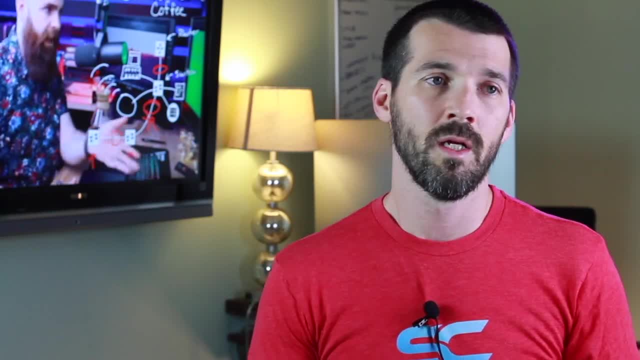 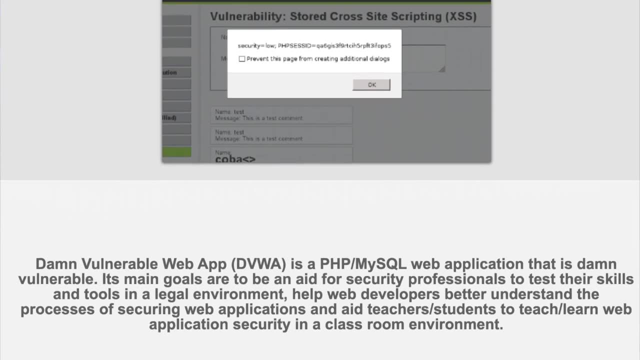 hard work in making it um accessible and good. so today we are going to be looking at building out the damn vulnerable web application. we're going to be building it out in aws, which is, if you've been following the channel for a while. you know that i work in aws for my home labs because it's 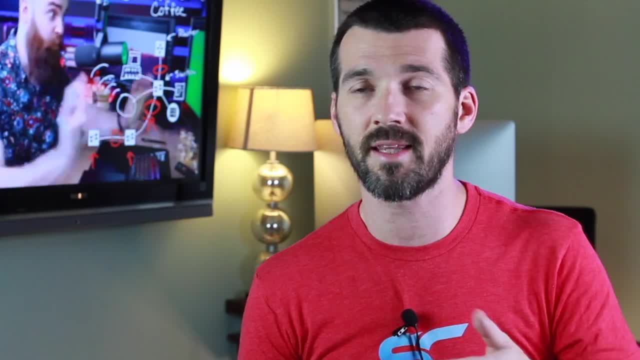 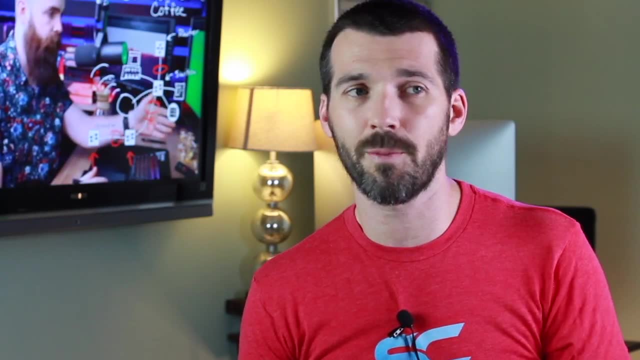 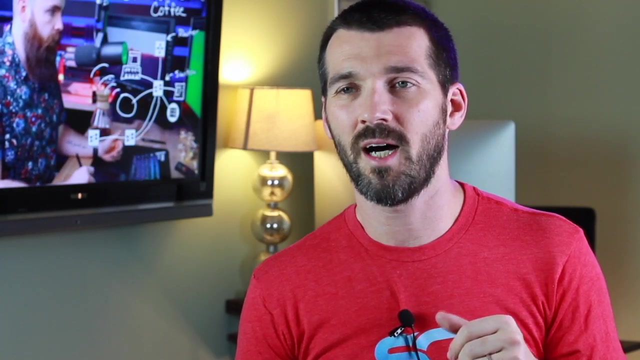 free. you can spin it up, spin it down. it doesn't cost anything as far as like resources and financial right. so, um, on juice shop and webgoat, we use docker polls. we're going to use docker today, but i couldn't get it as smooth and seamless and silky as the other two in the video series. 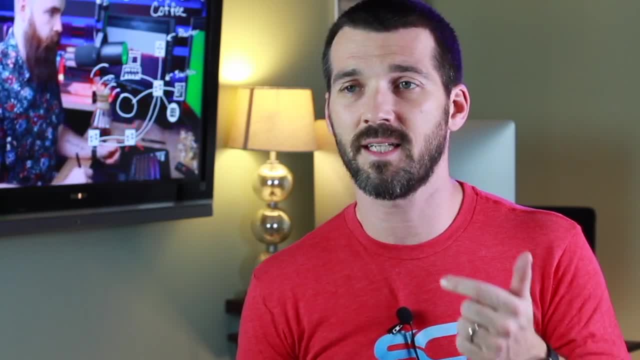 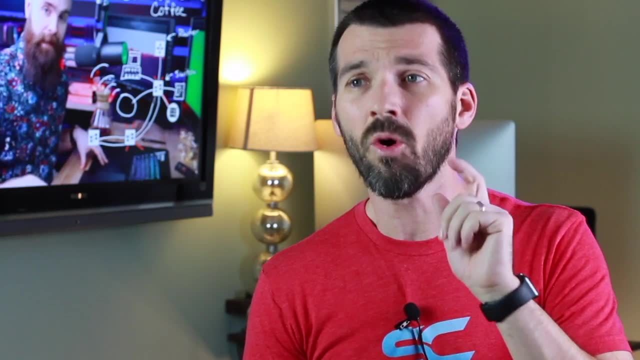 so we're actually going to have to secure shell into the box and uh, build it, uh, do the docker poll and everything so. but i will be showing you step by step how to do it. now why? why would you want to have vulnerable web application over the other ones? well, this one is. 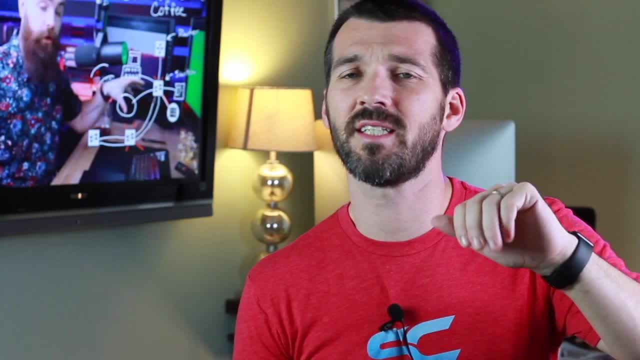 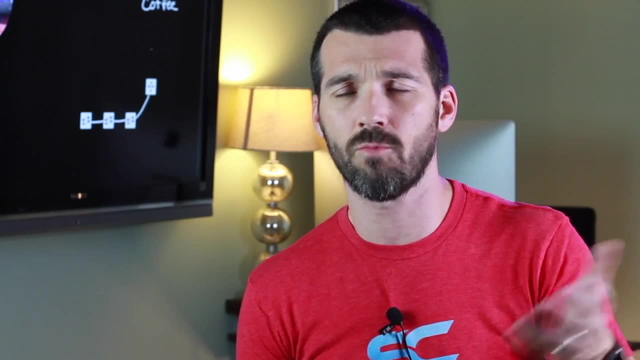 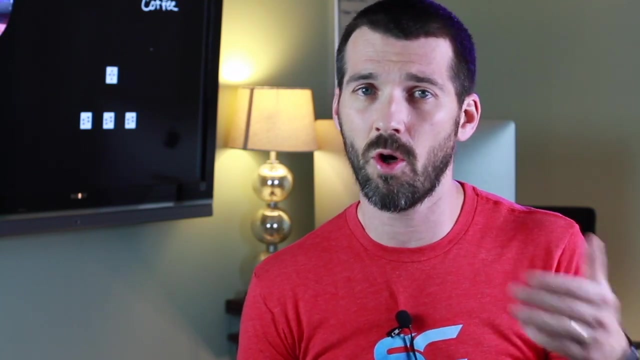 really well known, classic one. and what makes it interesting is you can actually kind of change the level of hardness, hardening on the- uh, the web application server itself. again, you're installing a very vulnerable web application. it allows you to execute, you know, operating system level commands at the os underneath the web app. so definitely be careful. 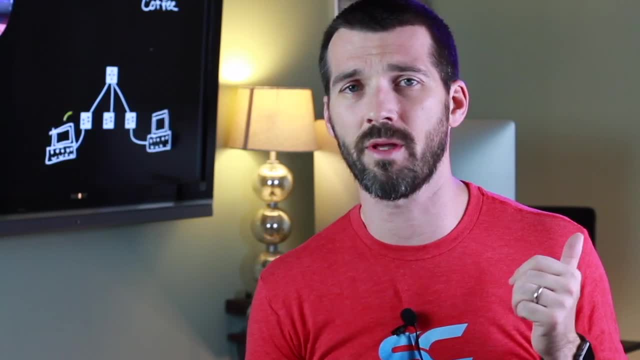 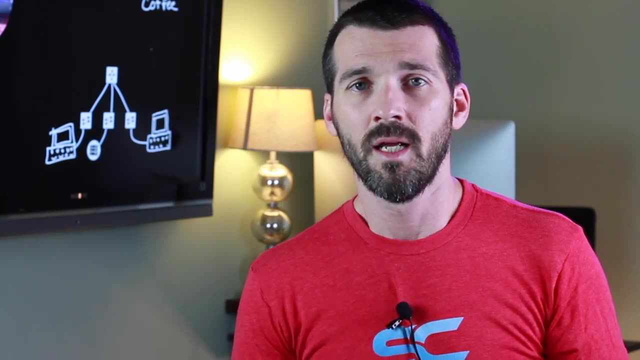 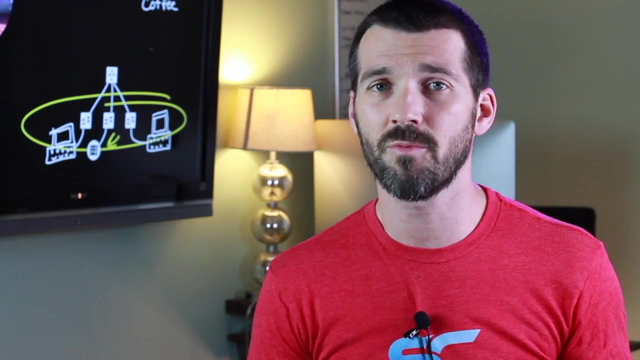 with how you deploy this and i'll show you, when we roll out the aws instance, how you can make it so only your ip address, uh, can access it. so, uh, just a little shout out: uh, we're, we're recognizing network chuck, another great information security youtuber here on youtube. uh, definitely check out. 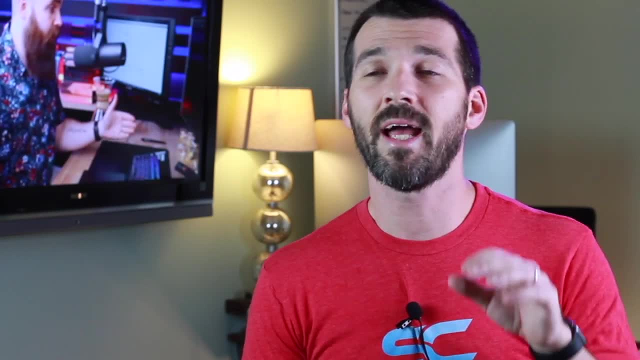 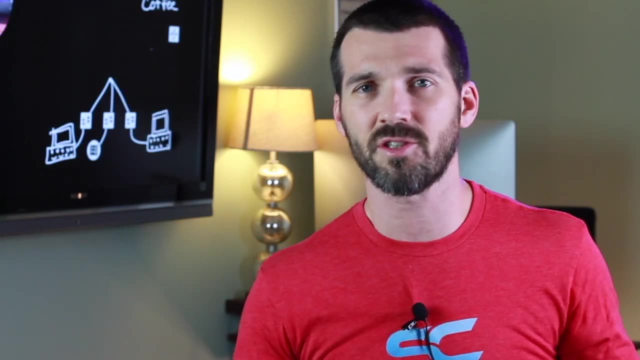 uh his channel, because he's got a lot of great content. okay, and, by the way, as i mentioned, this video is part of a series, so if you're interested in this, uh check out the playlist that's associated with this. uh, stefan waldvogel's uh list of different resources, because i'm basically 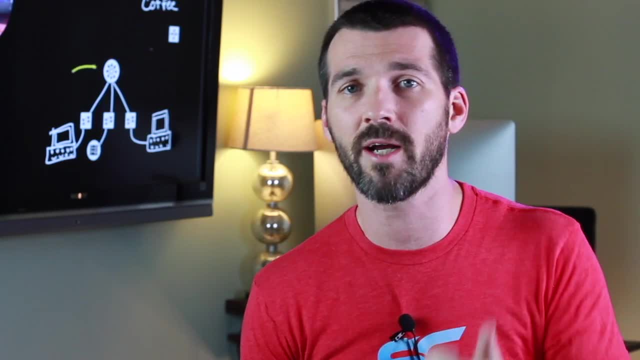 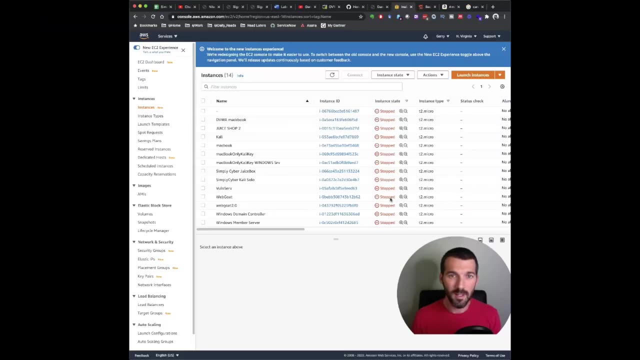 making them all. but let's hop behind the computer, build out our aws instance, get damn uh vulnerable web application up and get going. okay, let's go. hey, all right. so we're logged into our aws instance right now and if you need help registering for aws or setting up your billing, 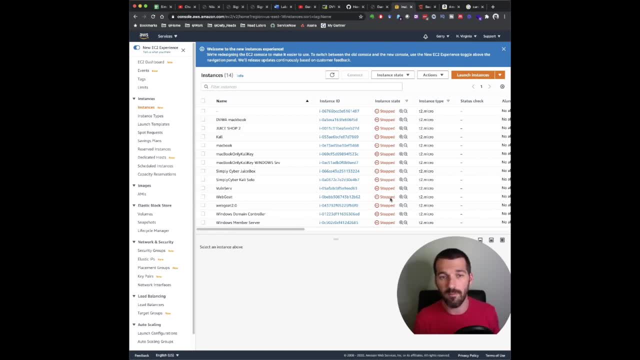 parameters. uh, check the show description below. i've put some comments in. i watched a video myself on free code camp on how to set the parameters and i've never had an issue. i've never had to pay in anything. so we're in our aws. we're going to go to services ec2. 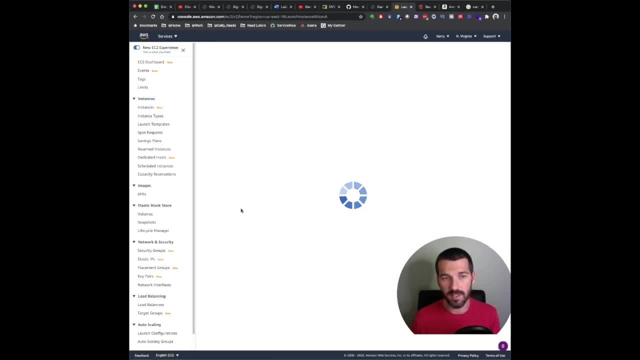 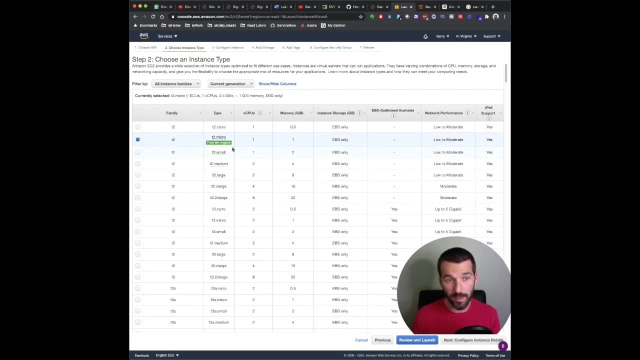 we're in here, we're going to launch an instance and we're just going to do our basic amazon linux 2, the very first one that they give you. go ahead, make sure you pick that free tier eligible so you don't have to pay anything now. normally, if you've been following the channel. 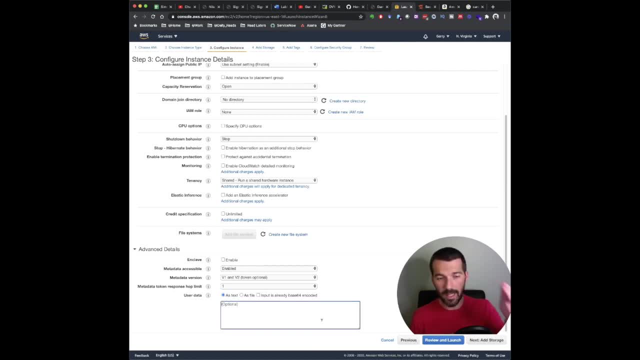 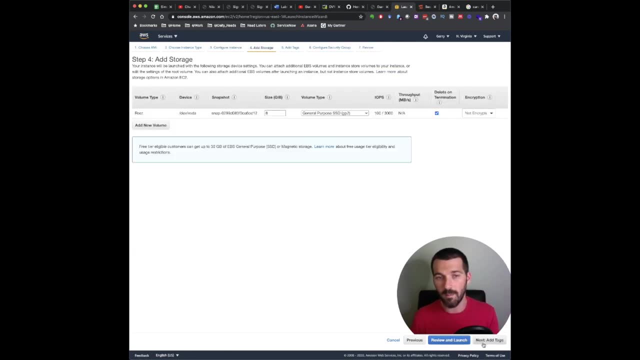 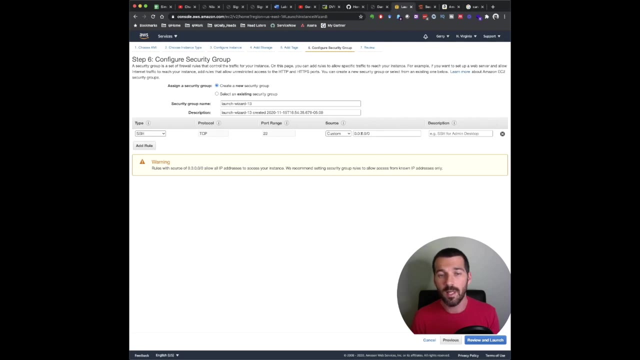 on the web goat in the juice shop, we would put our language down here in the user data section. that didn't work with the damn vulnerable web app, so we're going to do it a different way, a little bit more involved, but you know it's nice to get your hands dirty. make sure your ssh is open if you. 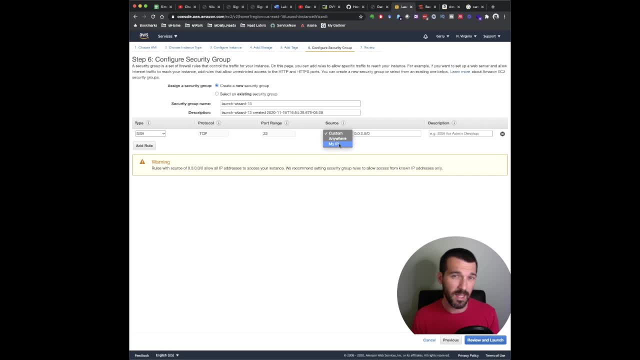 want to change it to my ip just to make it a little bit more secure, that's fine. i'm not going to do it for the demonstration and go ahead and add http port 80 and go ahead and do my ip if you want to keep it super secure, which i strongly encourage, or i'm going to leave it like this. 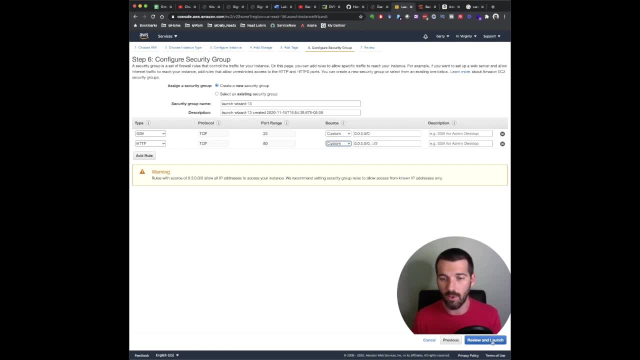 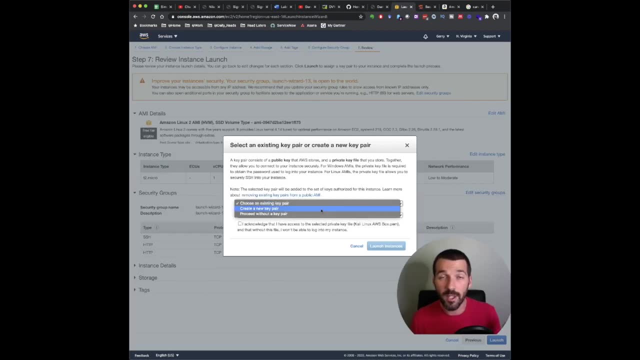 for the demo, because i'm going to destroy this right after i'm done recording. so let's review and launch now. if you haven't done this before, go ahead and create a new key pair. save that key off. it'll be a file, a pem file. you're going to use chmod to change the permissions on that um file. 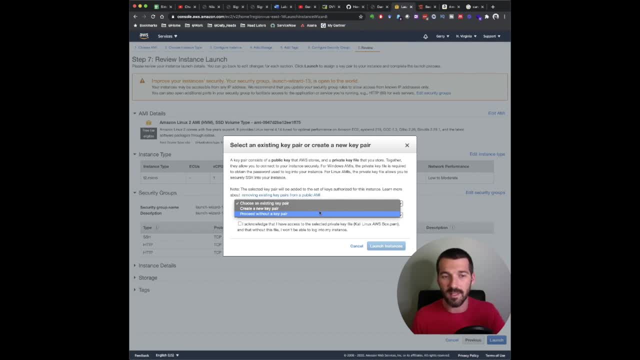 but just you know, if you, if you basically either created a new key pair or choose an existing one, if you, uh, have been following the show and you've been working through the labs, you already have a key pair. if not, create one and make sure that you set the permissions accordingly, so you 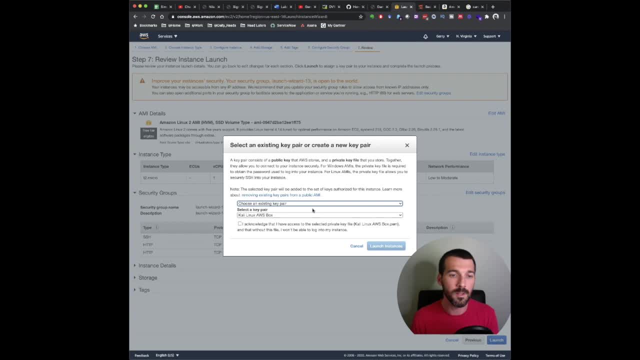 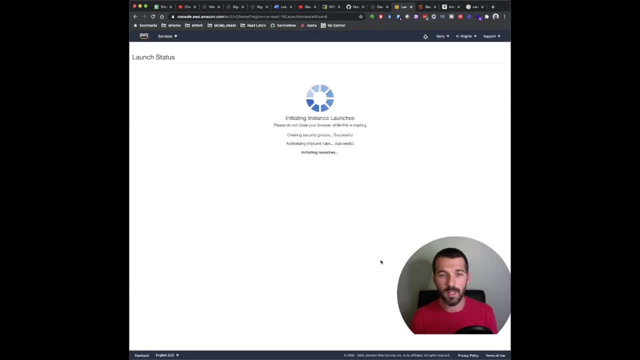 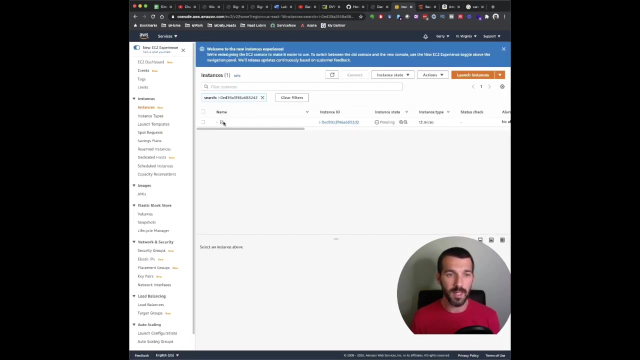 can log in, because that's what we're going to have to do. i'm going to use my simply cyber official key, hit acknowledge and i'm going to go ahead and launch it. okay, so, as amazon builds it up, i'm going to name this damn vulnerable web app. 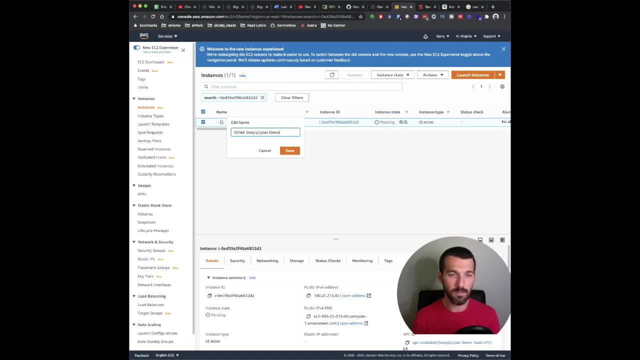 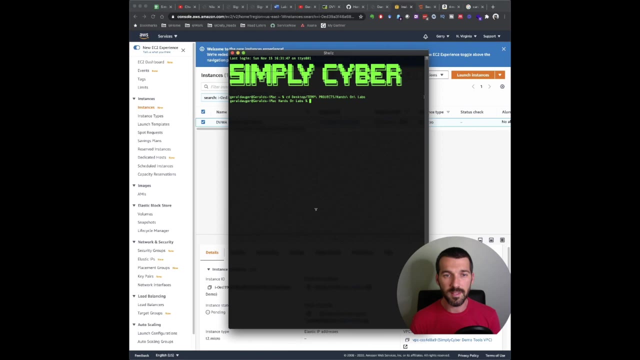 simply cyber demo. okay, we've already got our public ip, v4, dns, um url basically defined, so let's go ahead and, uh, you can see that i've already got um. this is the directory that has my uh dot pm file and again, you'll notice the permissions over here. 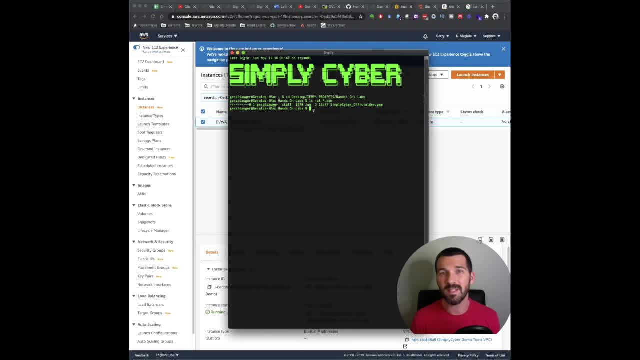 that they're set appropriately. basically, uh, amazon won't let you log in to your box unless you have the permission set correctly, so let us do ssh, dash i, the key ec2 dash, user at, and then, uh, paste the url. we're going to hit. yes, informed windows SCHNACK. 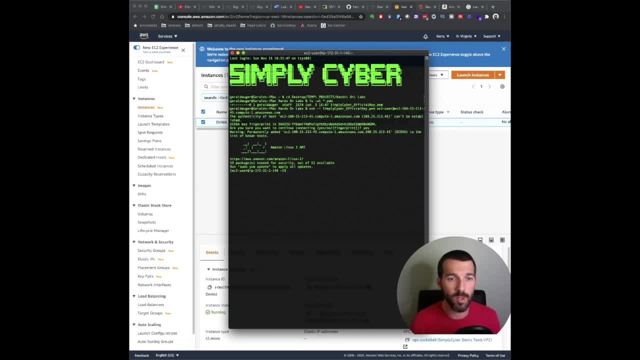 the server is being built right now and there we go, we're logged in. who am i? probably ec2, perfect, okay, so we're in our box now. now, normally, um, you would be able to just do this, uh, through that command, but because it didn't work, 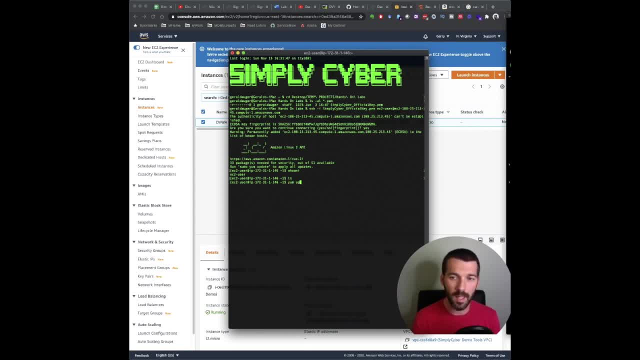 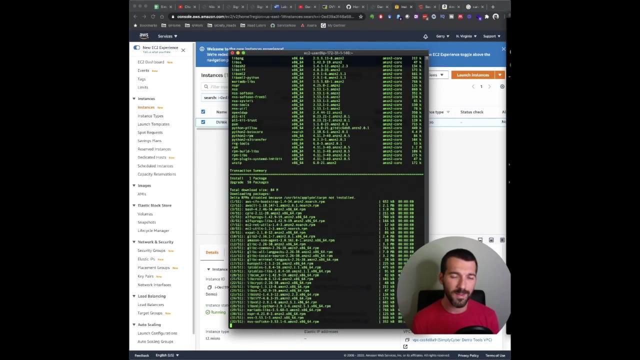 we're gonna do it this way. so do yum, update dash y, and i'm going to put this in the description below. so just check that out, but follow me, follow along with me. Oh, you have to do sudo yum, update dash y. I was doing this earlier. You could probably super user into root, but I don't. 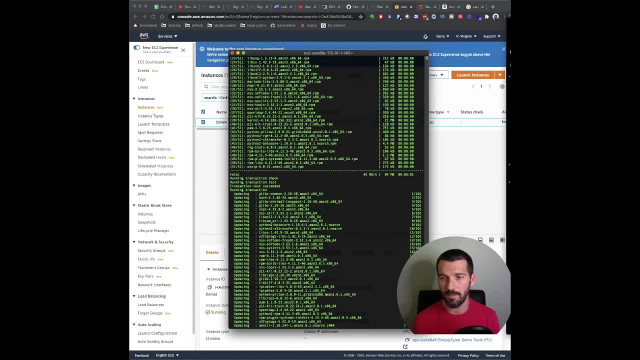 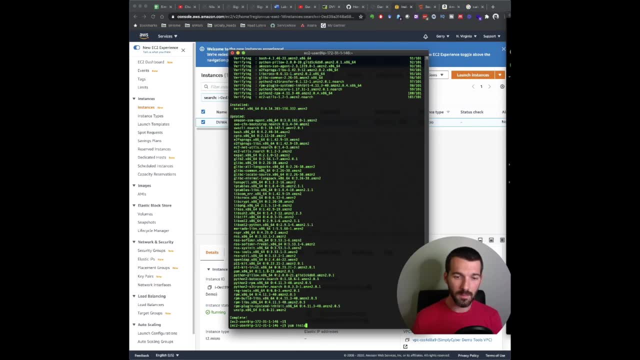 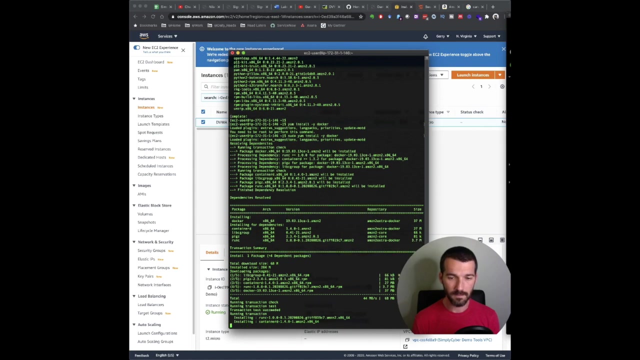 know what the root account is and I didn't bother googling it because sudo is going to work just fine. So I'm going to speed the video up here. We're going to run yum, install dash y docker. to install the docker application, again with sudo, because I keep forgetting. Now we're going to 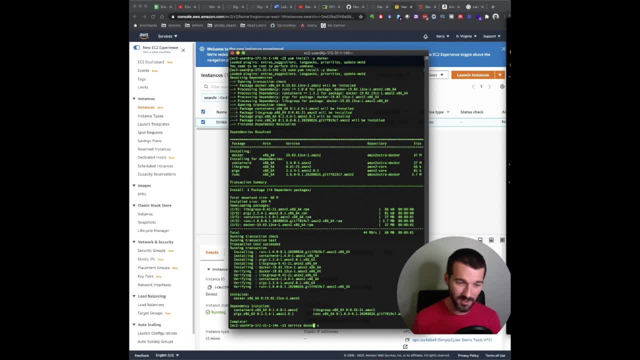 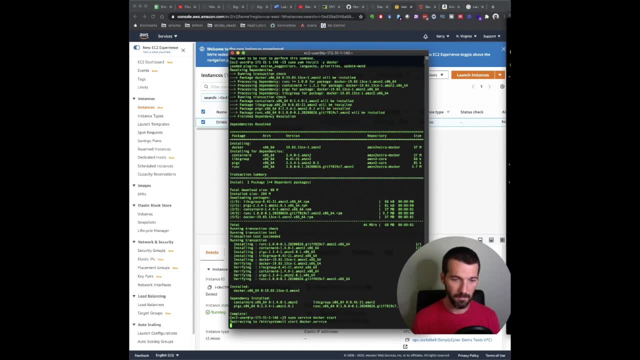 actually start the docker service with sudo. Don't forget the sudo. We're going to do docker run Tac, tac, rm, tac, tac, it, tac p 80, 80, vulnerable slash web, damn vulnerable web. 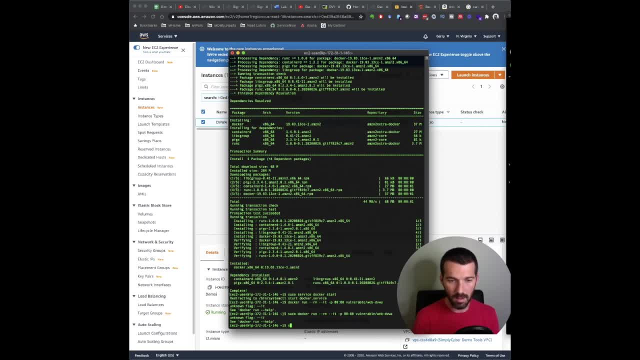 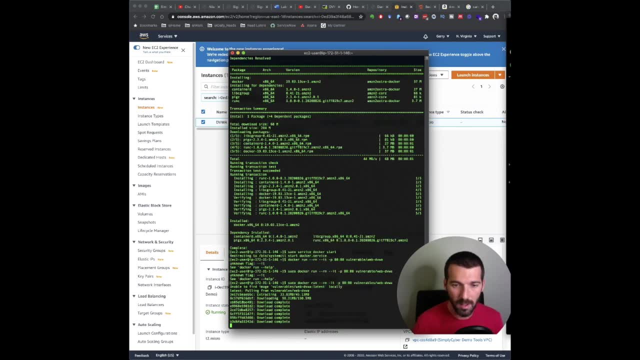 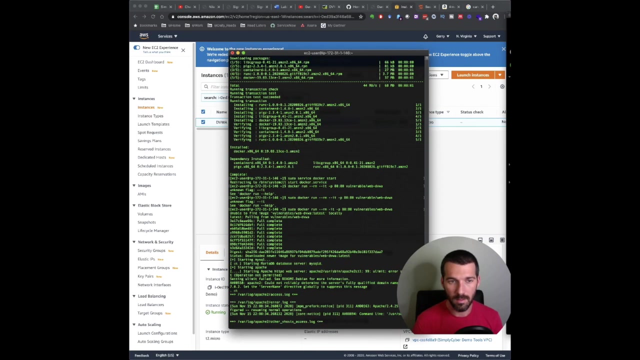 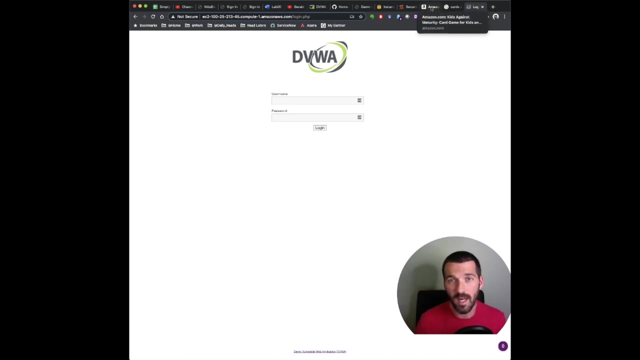 application. Okay, I don't know what it. I must have typed it wrong, but now we're running it. Oh, I did vulnerable, not vulnerables. Okay, let's fast forward. All right, there we go. So now we are logged in. I simply took the IPv4. 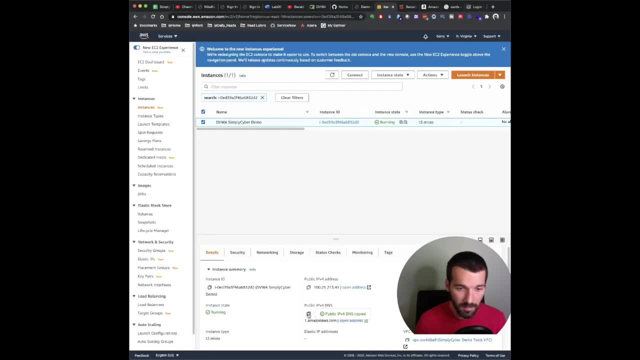 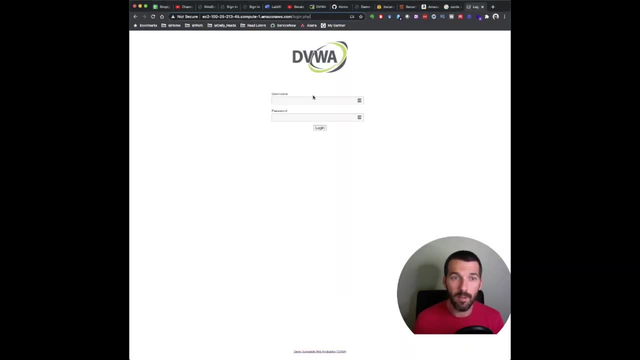 domain name DNS. after doing all that the docker, install stuff and running it, And here we are. We're presented with the interface to the damn vulnerable web application. Now I told you before, I'll tell you again: this is an incredibly vulnerable web app that will allow. 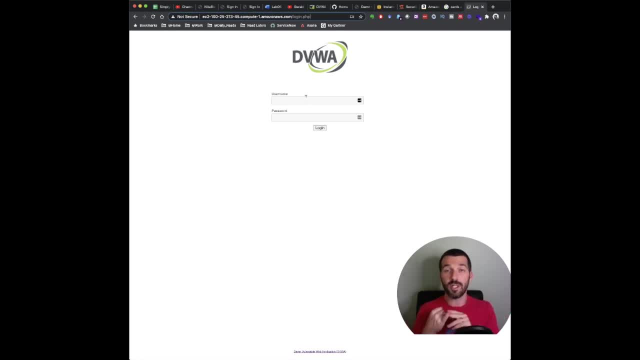 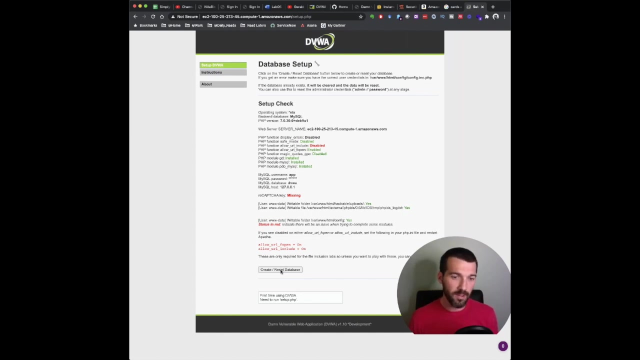 you to do a lot of bad stuff, So you definitely want this either shut down when you're not using it or constrained to only your IP address. Now, admin and password are the default credentials When you get in here. you're going to want to do the create reset database right off the rip. Okay, 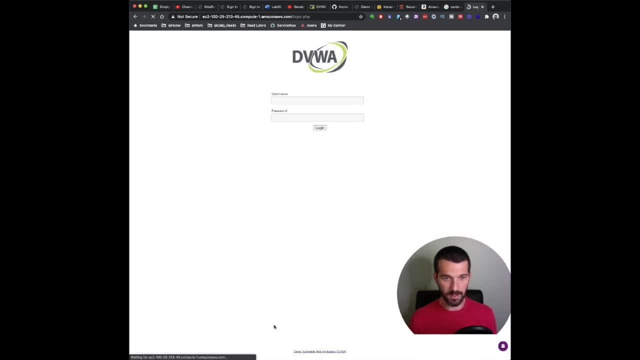 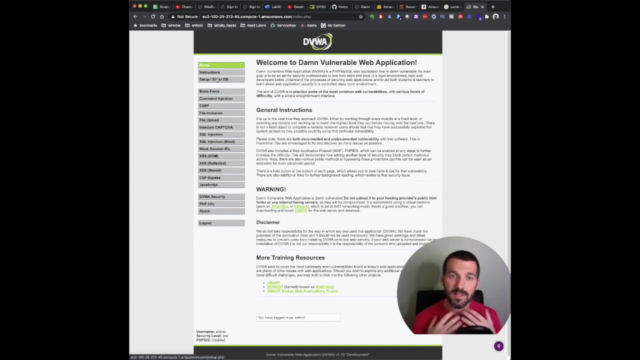 Okay, And please log in. This just kind of gets everything right and fresh. It's still admin and password, password And here we go, we're open. So now we are in the damn vulnerable web app. Now this is a great platform. 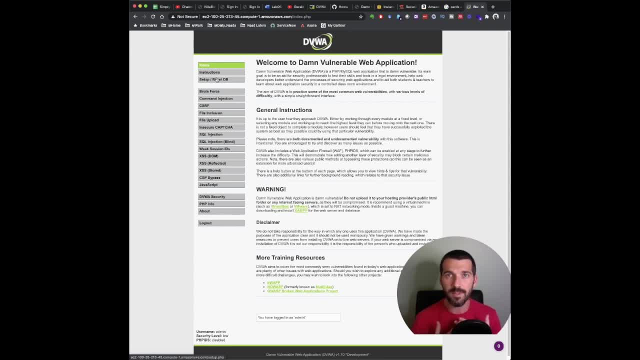 Again, it allows you to really learn the different kind of web application, type, vulnerabilities and how hacks are. You can see we got Crest site scripting both DOMs and reflected. We've got SQL injection. We have CAPTCHA, which I'm not even sure of, insecure CAPTCHA. I haven't done that myself. 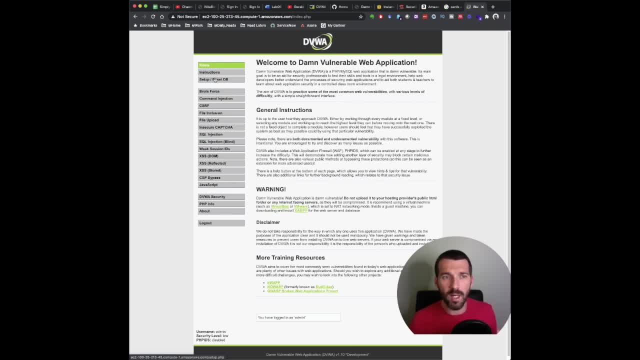 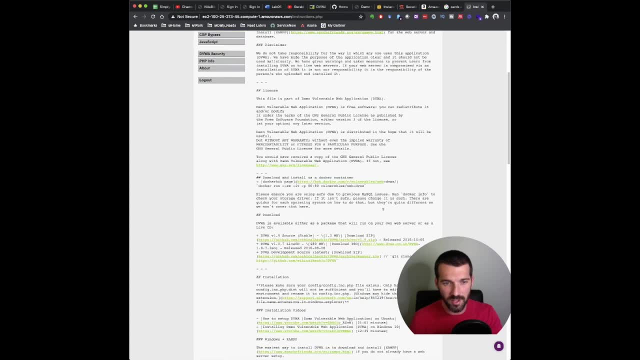 Command injection, which is great. Now I'll just stop for a second and say: you know, there's some administrative stuff, There's the setup right. They give you some instructions on how you can follow it, which is very nice. The DVWA security tab: I want you to. 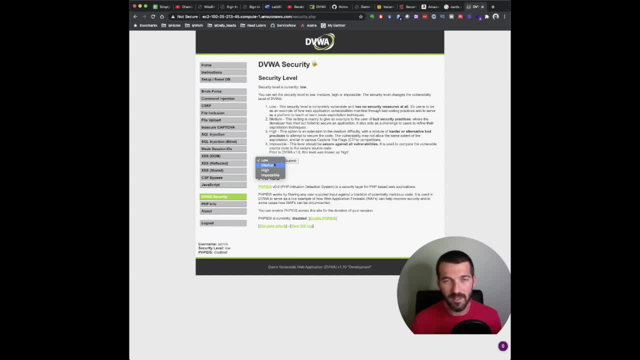 be aware of that, because this is basically kind of like a very, very easy way to harden or soften your target right. So I recommend that you start it low and kind of work through it. They give you a description here on what the different levels are, which is very cool. The PHP IDS is enabled. 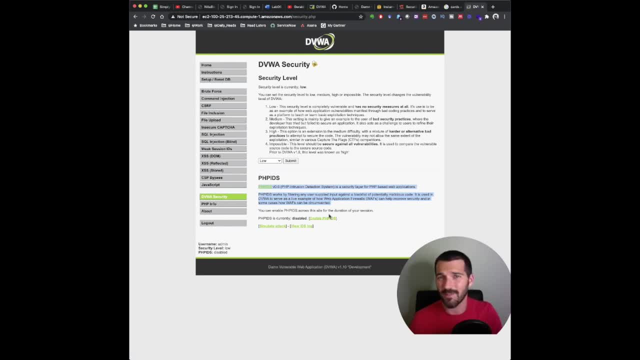 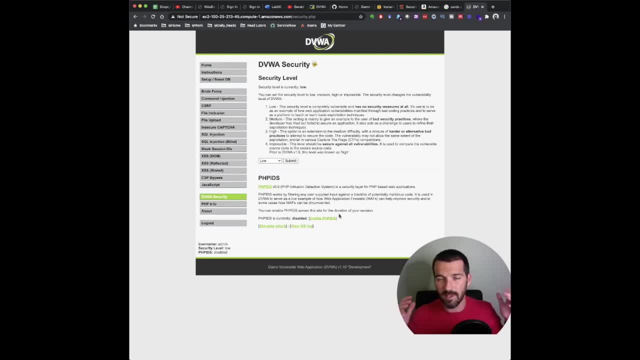 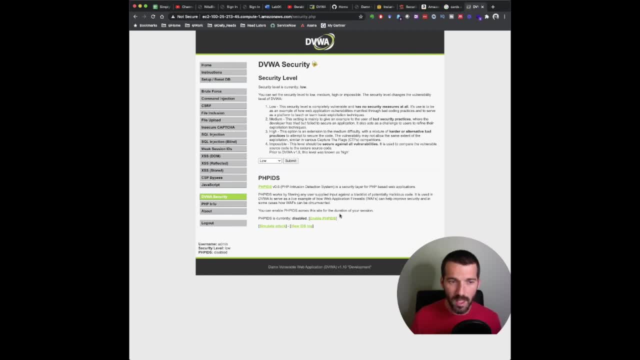 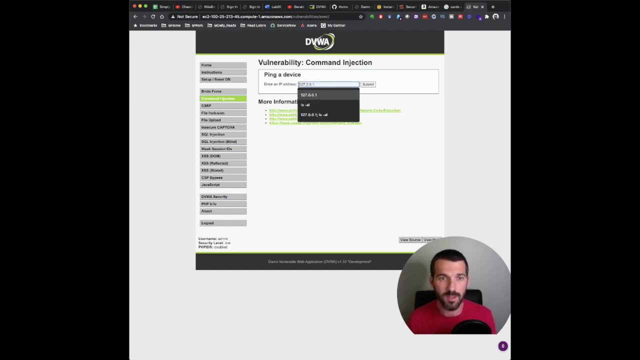 enjoying damn vulnerable web application. Now I'll just say that you know, just to give you an example, we'll do this, ping a device, So I'll do 127.0, right, This is local host, right. Submit. 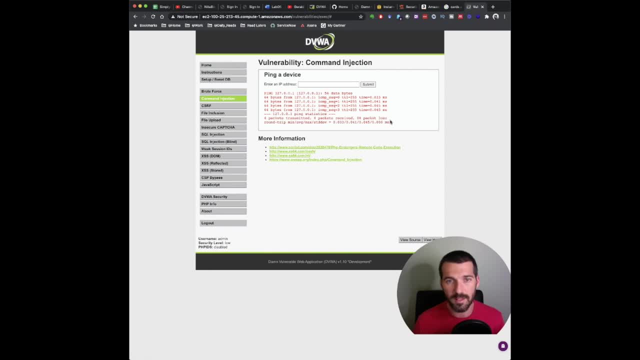 Here we go, We're going to ping it. It offers us the ability. This makes sense. If you've ever pinged from a machine like this is exactly what it looks like. So now let's see if it's open to command injection. So we'll say ls-al. 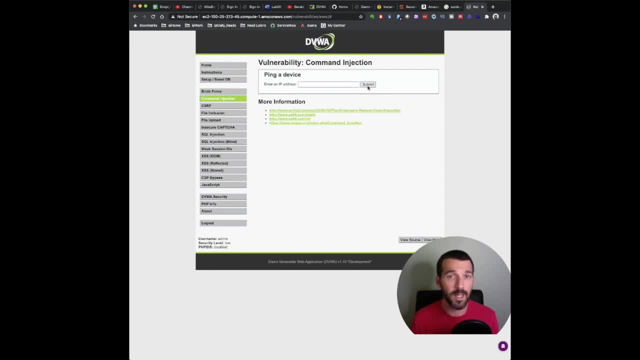 ls-al. Okay, It returns nothing. Now let's kind of combine the two. I've already done it here as testing. So we do the IP address and do a semicolon to terminate the command, Then we issue a new command, ls-al, And there you go. You can see already that this is a major vulnerability, right? So? 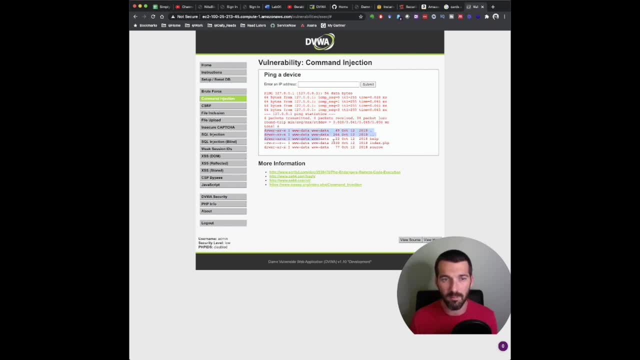 this is the output of the ping command. and then it ran my ls list directory contents Linux command. So this is not good. I'm basically executing commands at the operating system level. I don't know what the permission level is that's executing under. 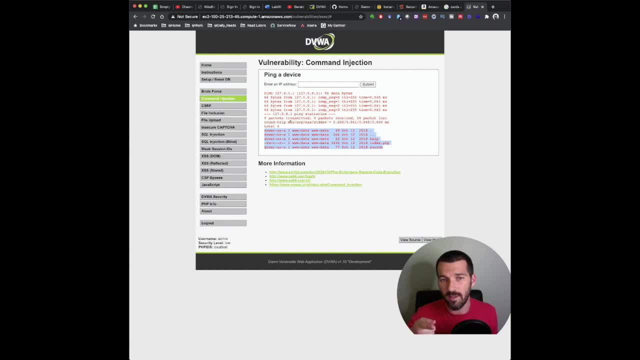 but the very next thing that I would attempt to do is create a user account and start to set it up, so I could then remote in over secure shell and start controlling it at the operating system level. So immediate circumvention. Anyways, the point is, this is very cool. Now they do give you some more. 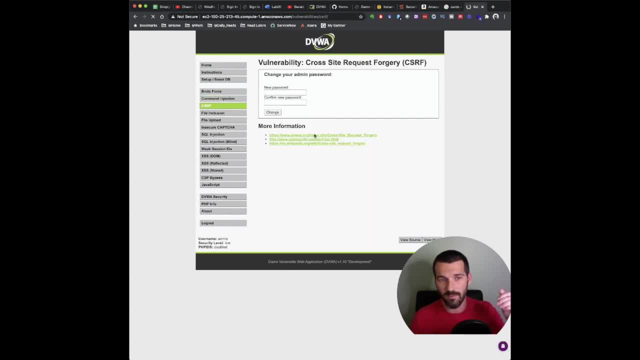 information for this particular exercise and you can see that they do it for the other ones as well. So you can kind of learn the concepts, learn the topic, et cetera. I didn't enjoy seeing the Scribd one because that is, I guess, a paid service. I clicked on it and said I could register for 30 days of access. 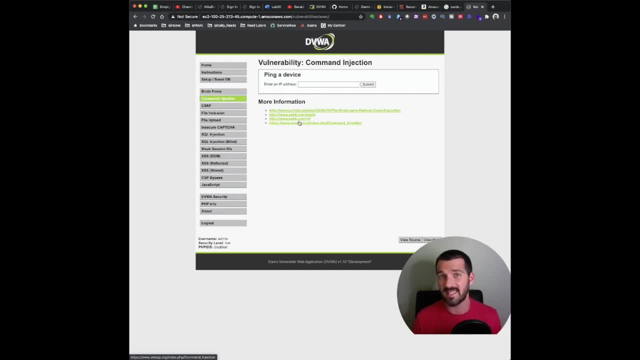 But these right here, these are not. OWASP is basically the go to nonprofit like ground zero resource for information around web application security, So I love that they reference that So you can use this platform a to practice and again learn how to execute a. 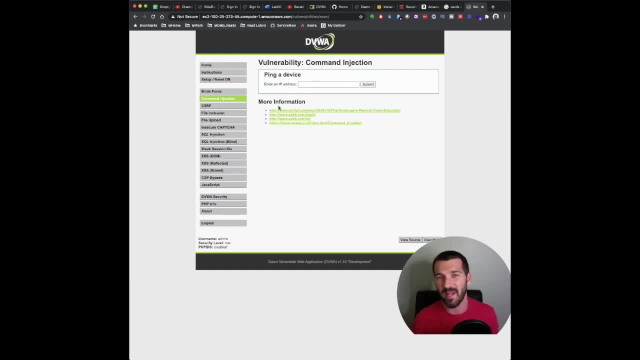 task and then what the attacks can look like and really give yourself perspective on, like, what's the scope and breadth of what an attack can do. like web application and I'm executing operating system commands. That is really not a good idea, right? Like that's definitely not the intention of whoever designed the web. 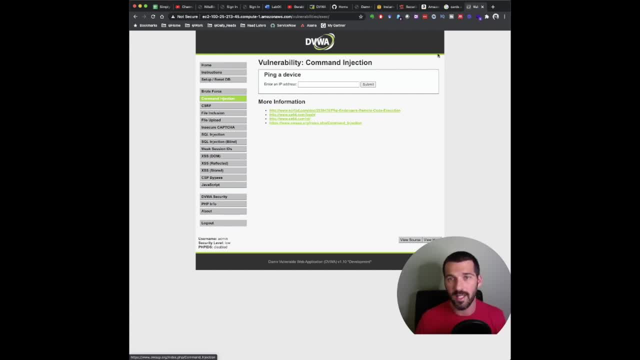 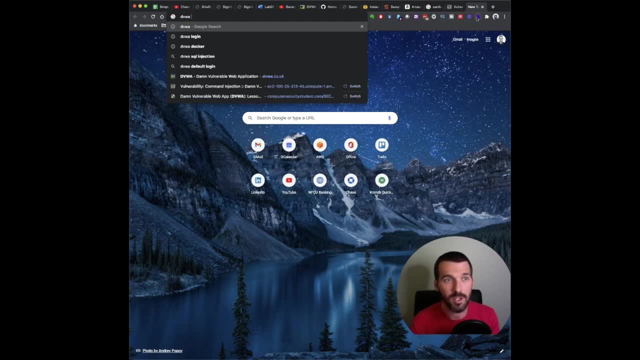 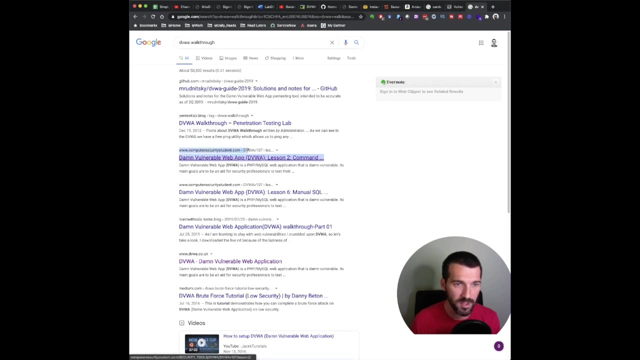 application. So definitely cool, Definitely worth checking out. I also want to share that there is a damn vulnerable web application walkthroughs. I did some research and I found I think it was this one right computer security student dot com and I'll link to this in. 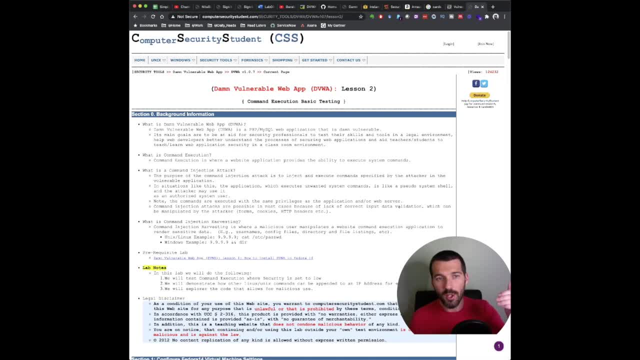 my show notes. They actually walk through all of these and they have it built. I also teach on the side and they have this built like a lab that you would get in a regular kind of higher ed curriculum with lecture and in lab associated, And I really enjoyed it So I wanted to represent it. I do want to tell you 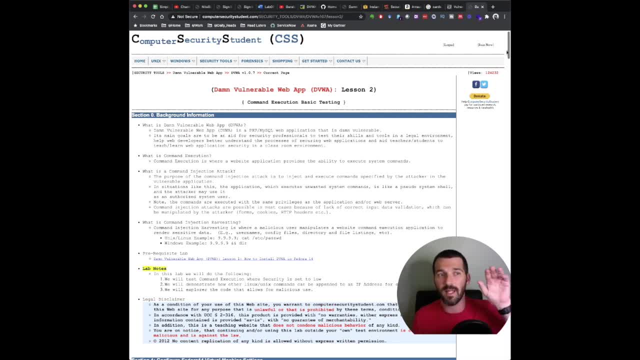 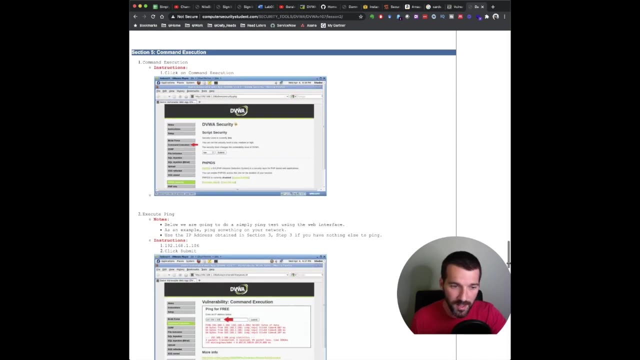 that this is not the same as building it in a WS, like the computer security student builds it in a Fedora Unix instance, which you don't need to understand. all you need to do is that you're not going to see all the Amazon stuff just jumped down to the part where they're actually doing the lab, right like boom. This is the same one, right? 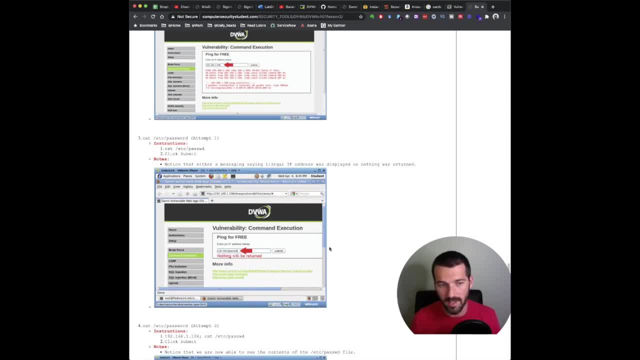 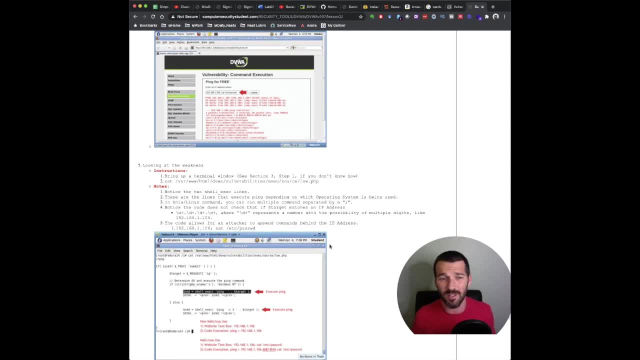 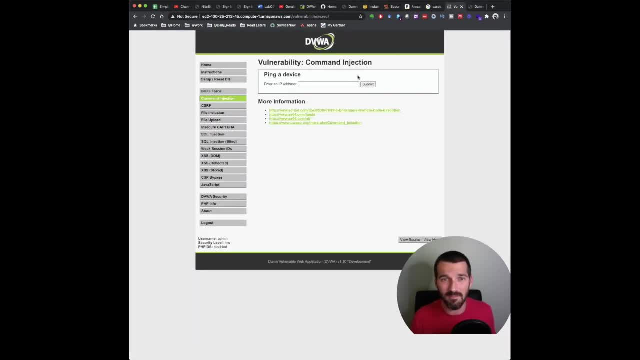 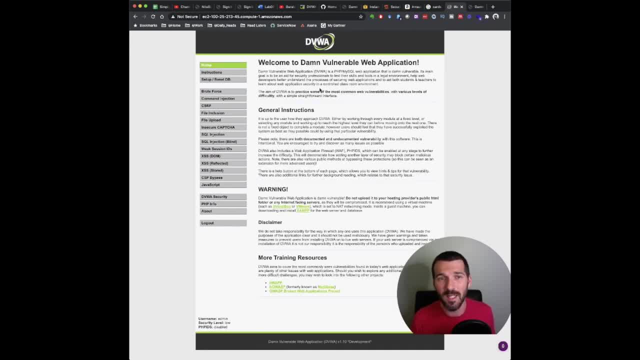 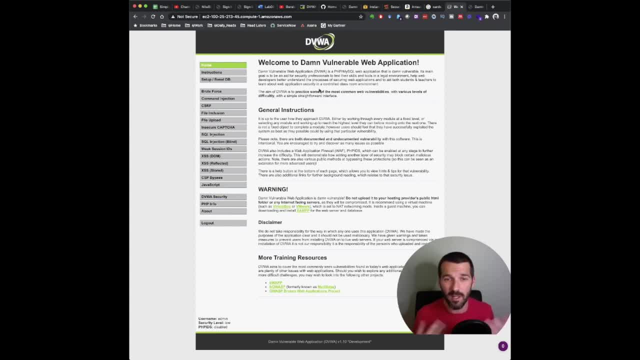 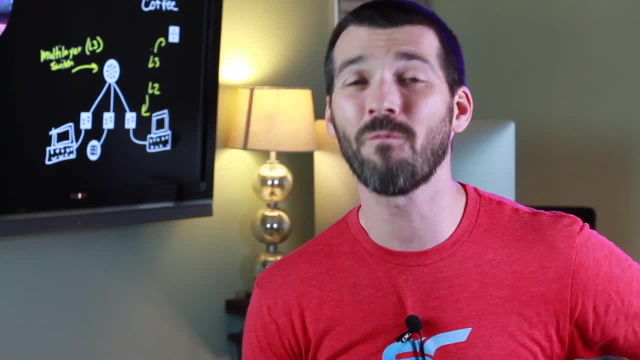 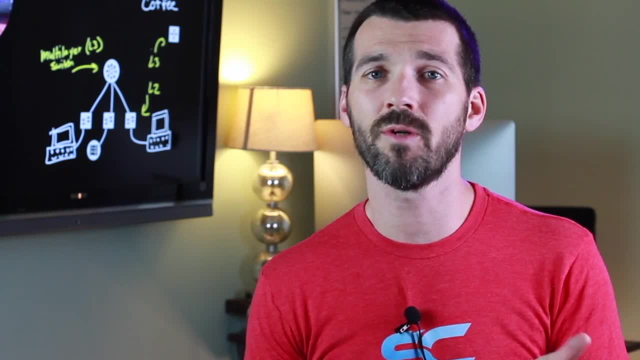 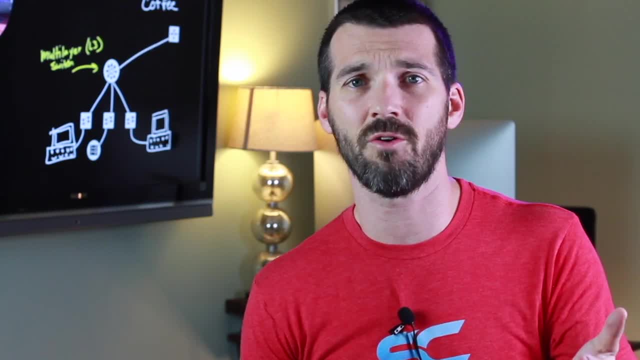 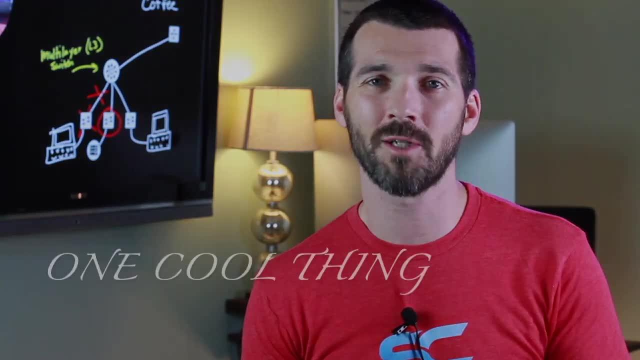 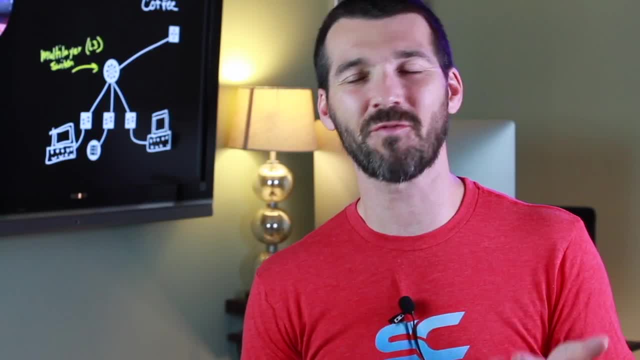